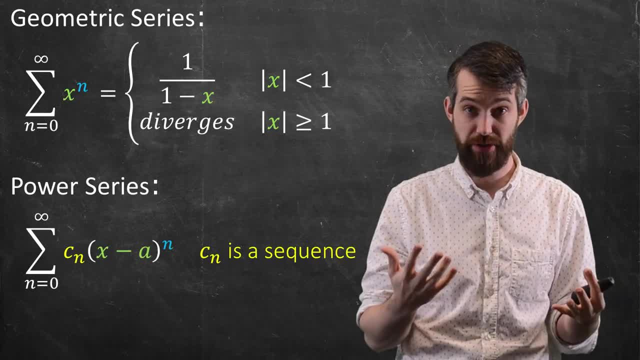 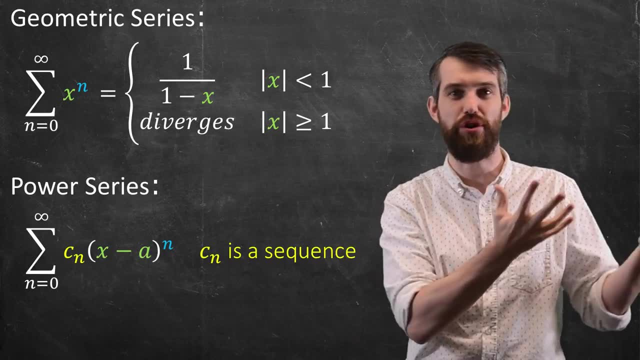 Something that we call power series. So a power series is like a geometric series in a couple different ways. Instead of x to the n, I'm going to have x minus a to the n. That's not so very different, it's just sort of a shift. But I also multiply it not by 1 every. 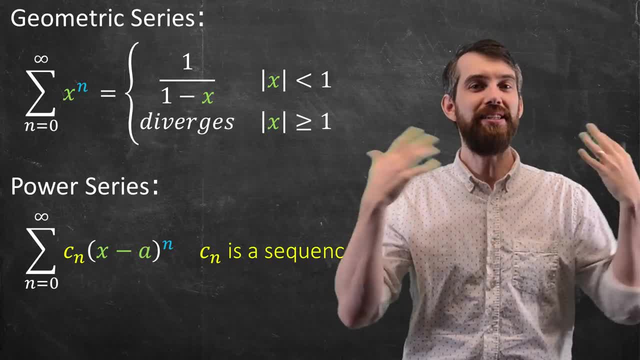 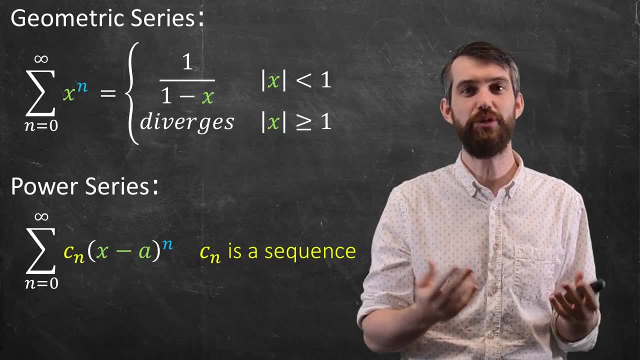 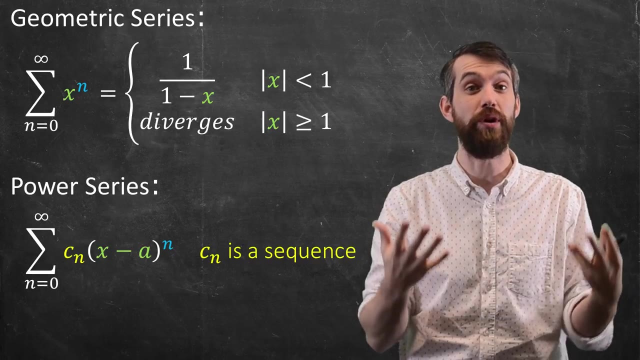 time, or by a constant a every time, but by an entire other sequence: cn. cn could be 1 over n or n factorial or who knows. So a power series is when you have a variable x raised to power of n And then multiplied by a sequence of constants like 1 over n or 1 over n squared or whatever. 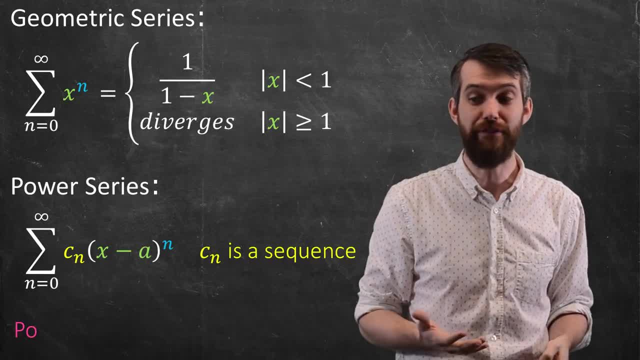 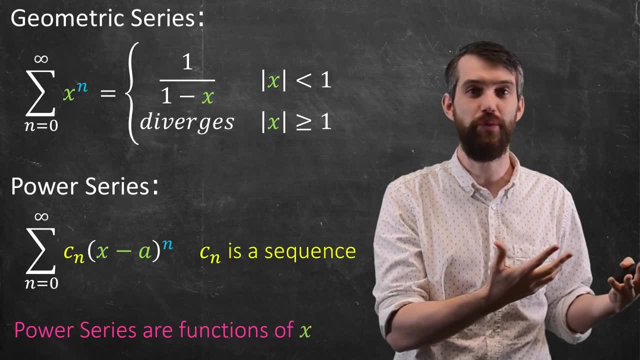 you like. Now the point is this: power series is a function that if you put in different values of x, you may get convergence, you get a value out of it, or it may diverge, in which case the function is not defined for that value of x. But either way it's a function. 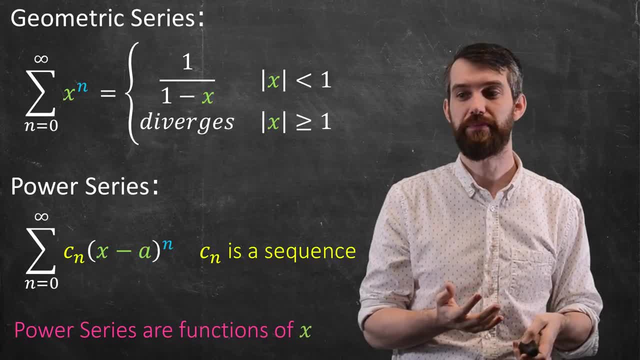 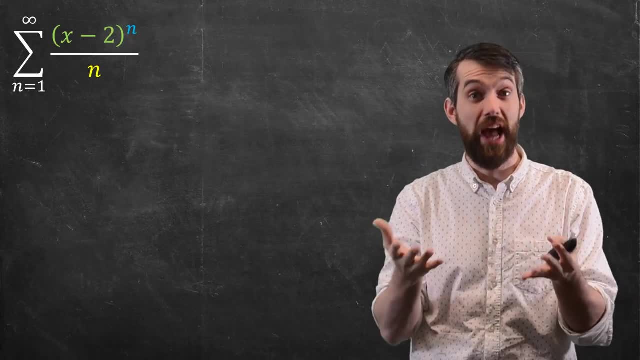 of x with some domain that we want to figure out. So, for instance, let's make this concrete by considering a specific example. In this example, the cn, that constant sequence is the sequence 1 over n. Then I have an x. 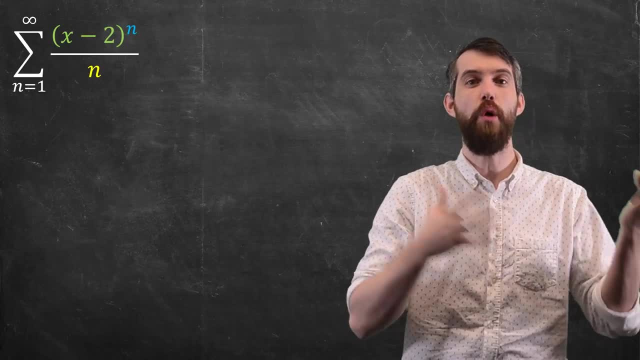 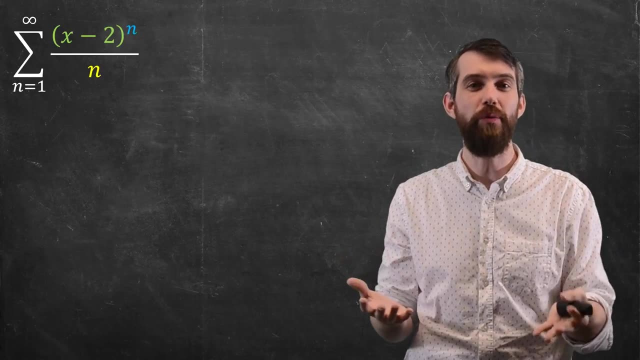 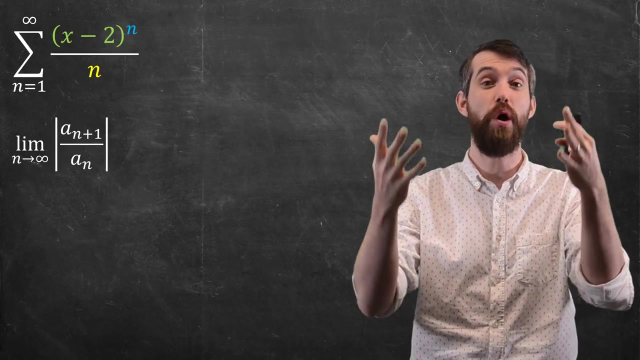 minus 2 to the power of n. Now, depending on what the x is, this may converge or it may diverge. It depends on that value of x. So how can we decide whether this diverges or converges? Well, we have the ratio. test this ratio of an plus 1 over an. You put the 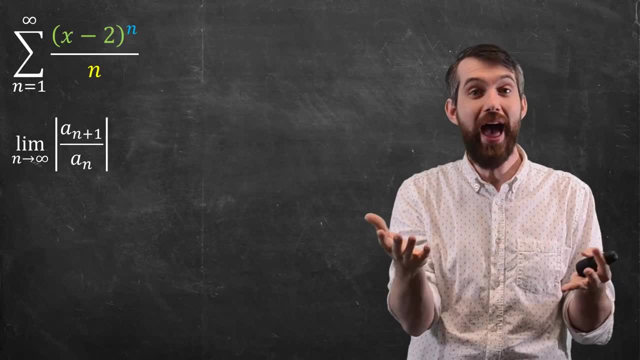 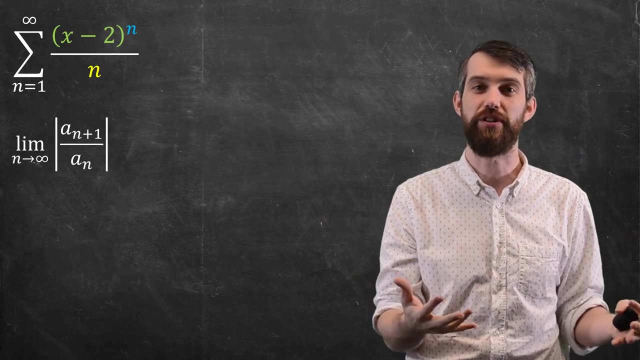 absolute value. take the limit as n goes to infinity. We can do that, and it will tell us when this converges and when it doesn't, What values of x make this converge and what values of x make it diverge. Okay, so let's plug this in. If I plug that into my ratio, on the top I have the an, but 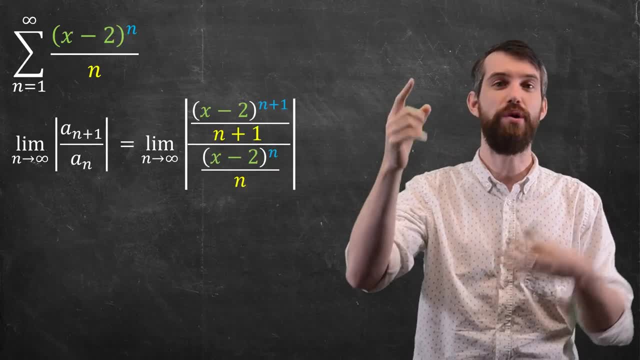 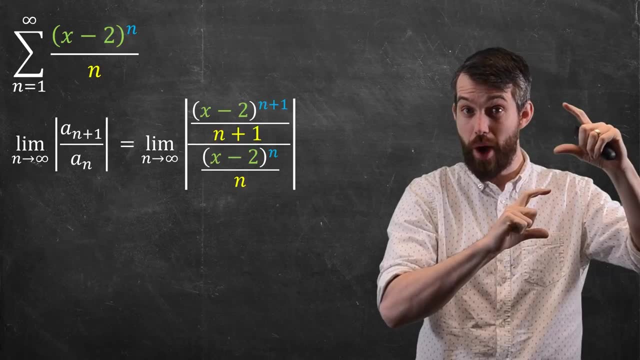 I put an n plus 1 everywhere, So x minus 2 to the n plus 1 over n plus 1.. And then I divide out just by the an. I have a quotient of quotients, so I'll bring the bottom one. 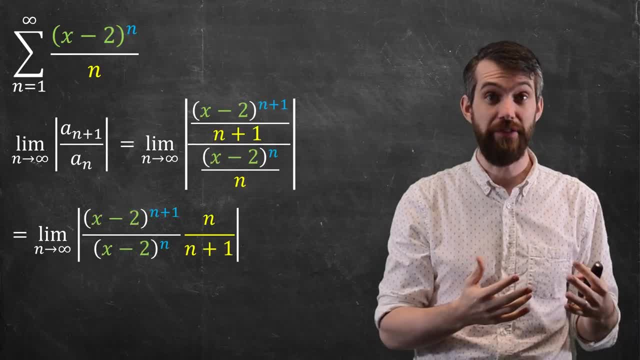 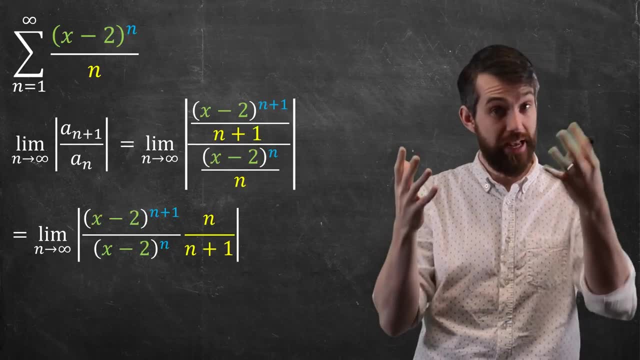 up, And what this is just going to give me is the limit of an x minus 2 to the n plus 1 over x minus 2 to the n, and then multiplied by an n over an n plus 1.. That's what I get. 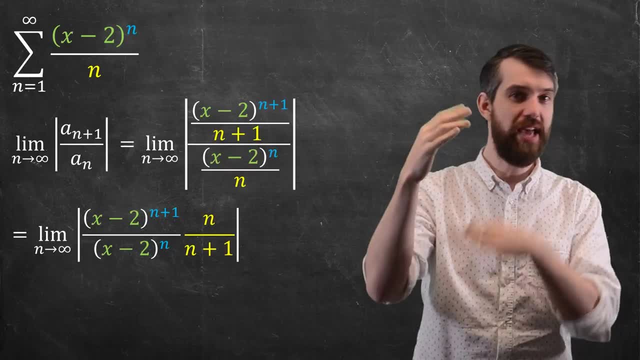 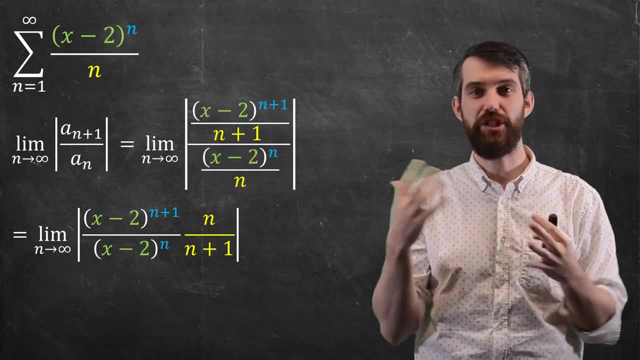 when I bring it up Now for the yellow, the n over the n plus 1, as n gets very large, that is just going to go to the value of 1.. Then for the x minus 2 portion, because it's 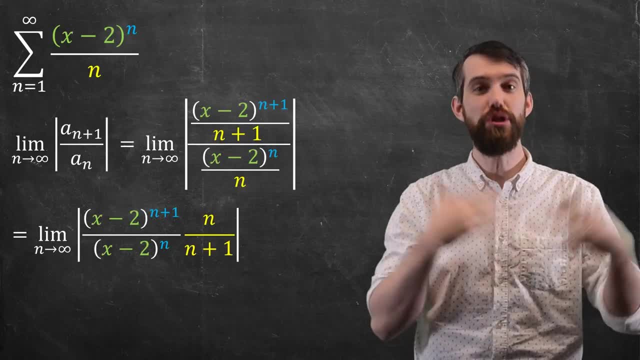 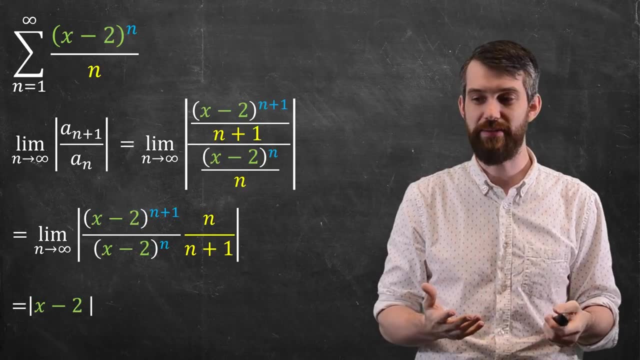 x minus 2 to the n, plus 1, and then x minus 2 to the n. most of those cancel and I'm just left with a single copy of this x minus 2 multiplied by the 1. So simplifying a little. 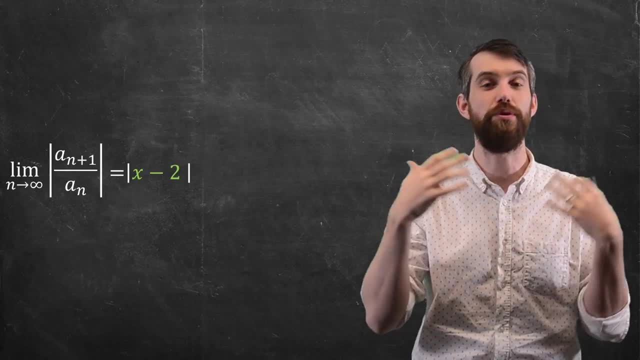 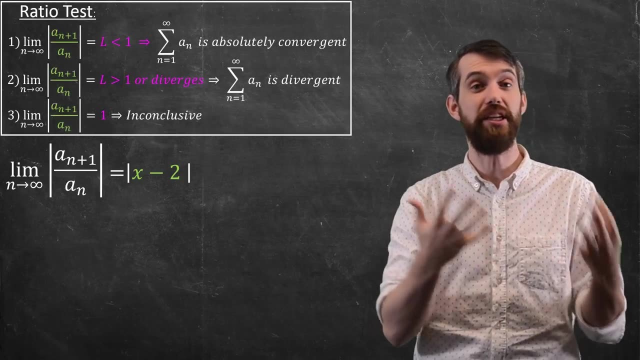 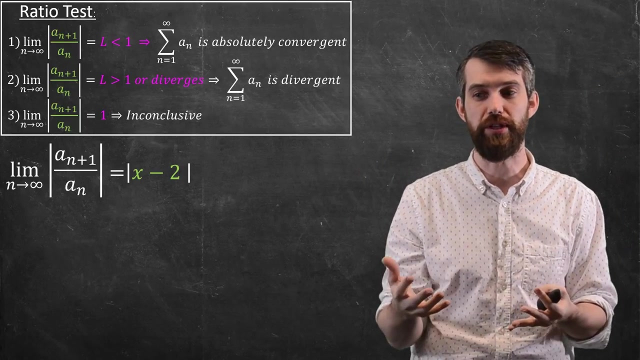 bit. I have my limit of my ratio And I'll remind you that what the ratio test told us is it gave us conditions for when that ratio was going to imply that the series converged absolutely, or whether it diverged or whether it was inconclusive. So if this ratio is less than 1, that's when. 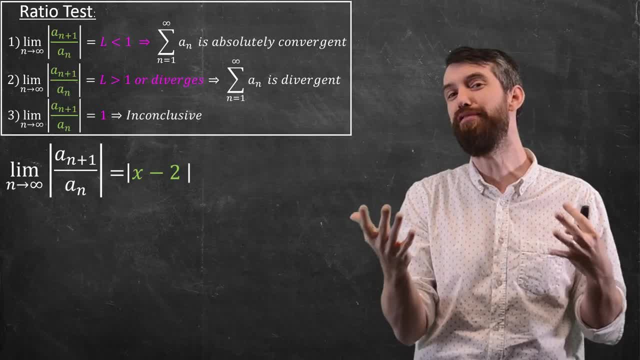 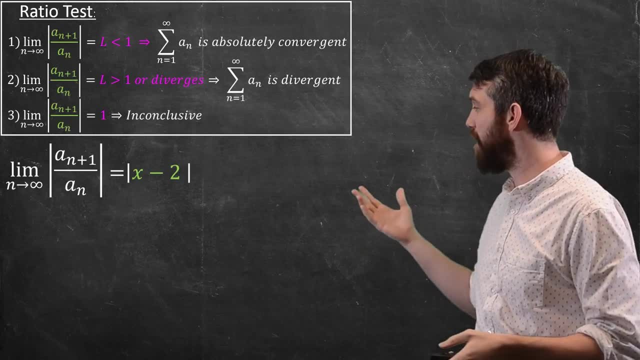 it's going to converge. And if the ratio is equal to 1,, well, it might still converge, but we'll have to do more work. We don't yet know from the ratio test, So let's do this. We know that our ratio goes to x minus 2.. So if it converges, that means it's going. 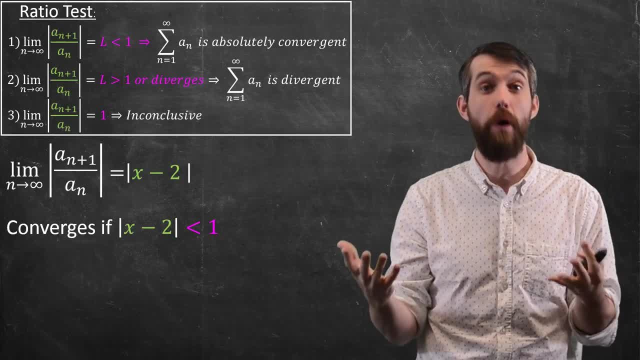 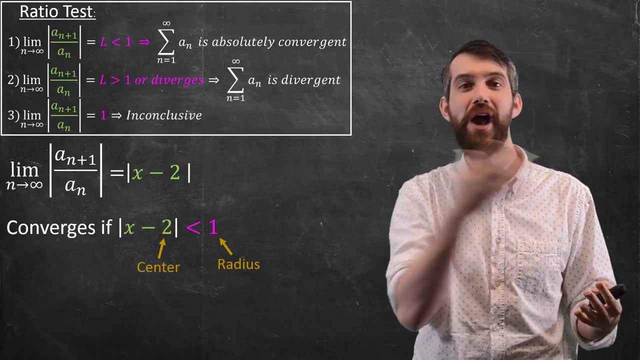 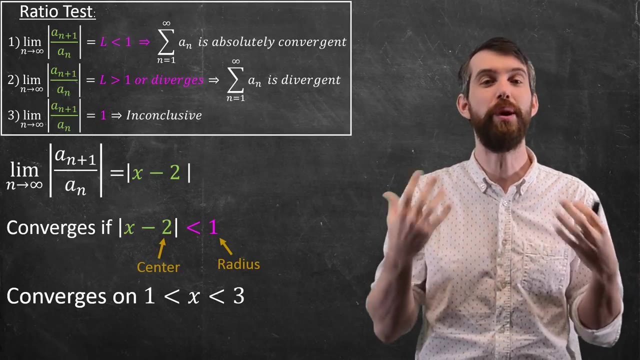 to be x minus 2 is less than 1.. This is an inequality with an absolute value. It has a center of 2, it has a radius of 1, so it's all points that are 1 away from that center of 2.. Which is to say that the ratio test is telling us it converges. if we are on the 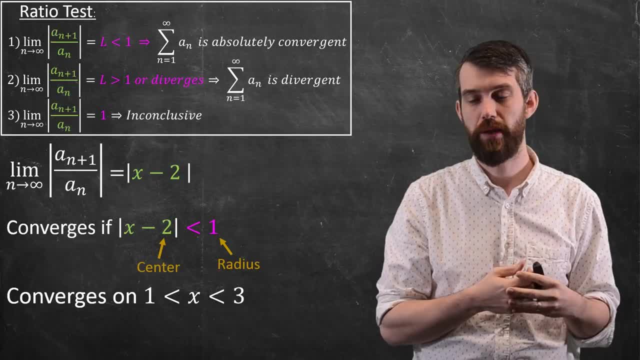 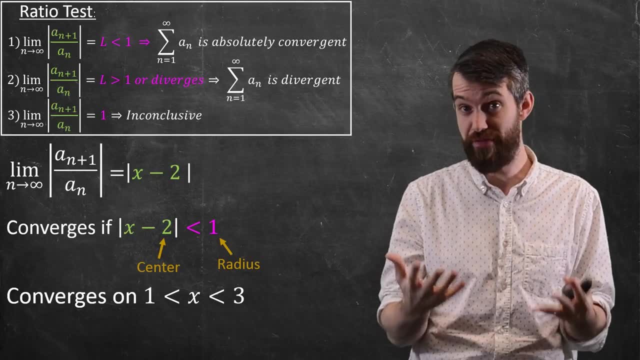 interval from 1 up to 3.. Now that is when the ratio test guaranteed it converges. Now that is when the ratio test guaranteed it converges. But it might converge for even more values of x than that, because there's also the inconclusive. 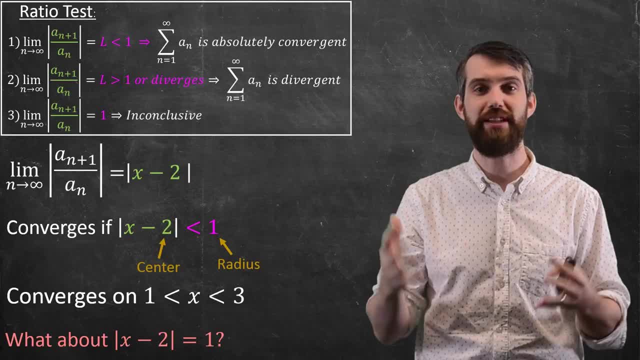 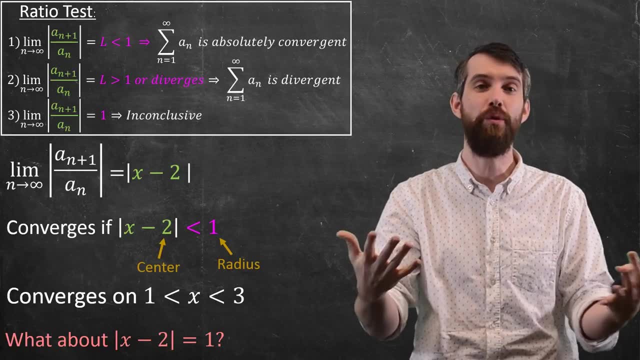 case. So how do we deal with that? What happens when the absolute value of x minus 2 is not just less than 1, but equal to 1?? Indeed, it's possible that it also converges there. If it's greater than 1, the ratio test says for sure: it's going to diverge. 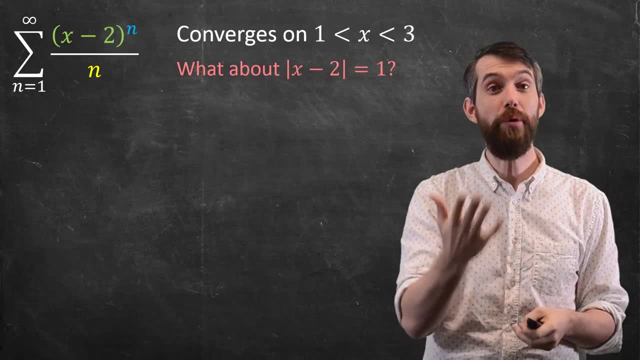 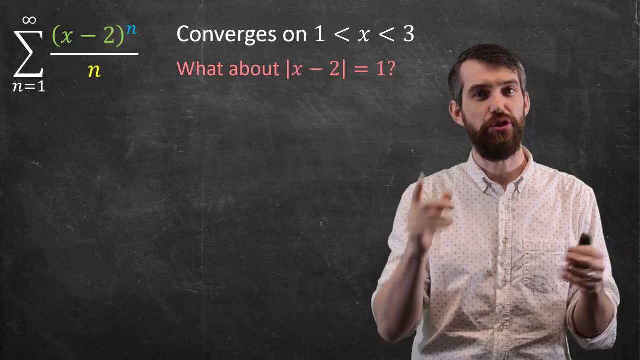 So let's go back to our original series, and we already know it converges on the 1 up to 3.. We want to see if we can do better than that. Now. when the absolute value of x minus 2 is equal to 1, this occurs at two different 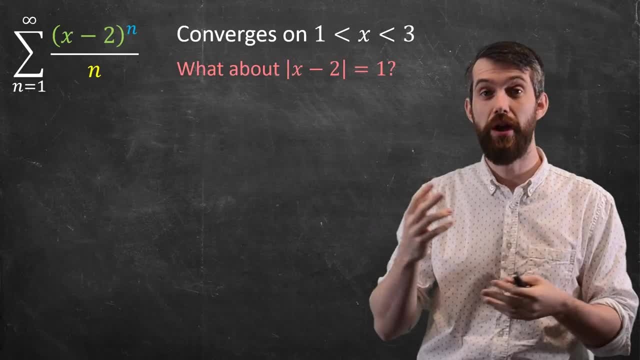 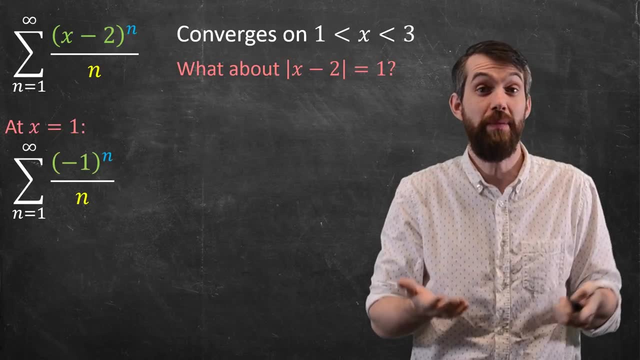 times, If x is equal to 3,, the one endpoint, or if x is equal to 1,, the other endpoint. either of those are going to take the absolute value and make them equal to 1.. So let's try just plugging them in. So if I plug in, for example, x equal to 1,, well, 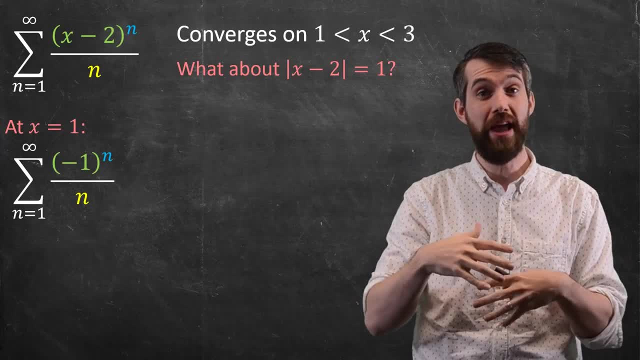 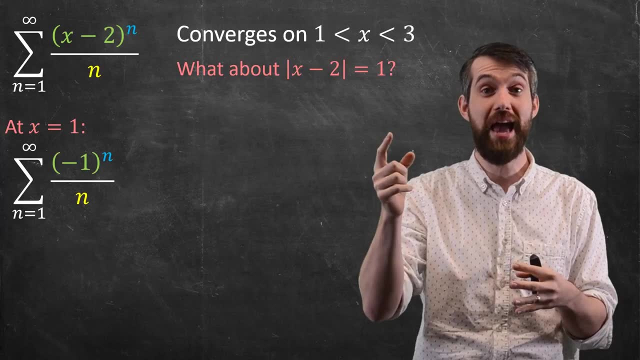 what do I get? It's minus 1 to the n over n. That's a series we've seen before. That's an alternating series. This is a series where you've got the minus 1 to the n multiplied by the positive sequence, with limit 0, this 1 over n, So this converges by the alternating. 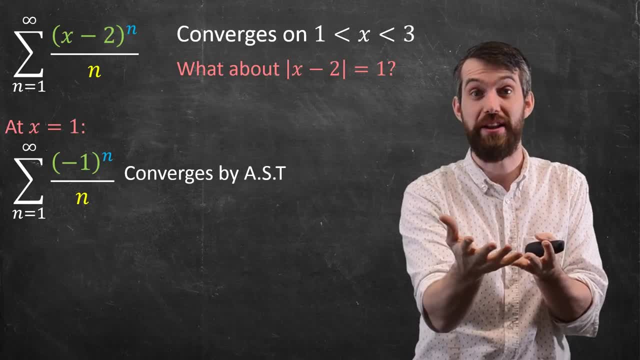 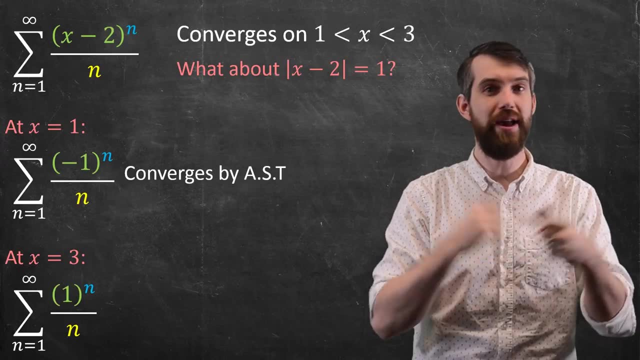 series test. So indeed, it's not just less than 1. here, in our domain, where it converges, It's less than or equal to 1.. But what about the other side of this? Well, if I plug in x equal to 3,, 3 minus 2 is 1.. 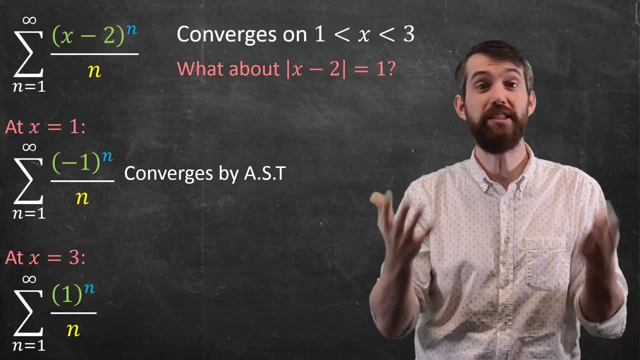 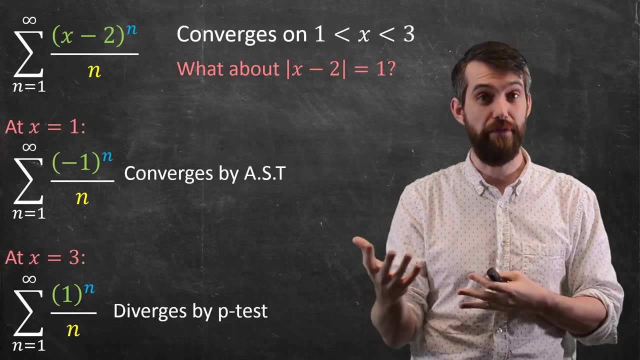 1 to the n is just always 1.. So this is the sum of 1 over n, which is a p-test. It's the harmonic series. This diverges, So on the one endpoint it converged On the other. 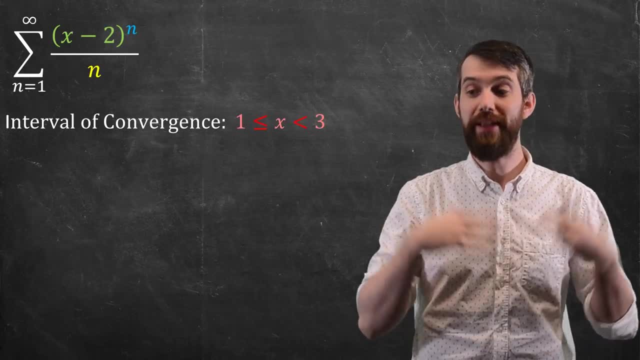 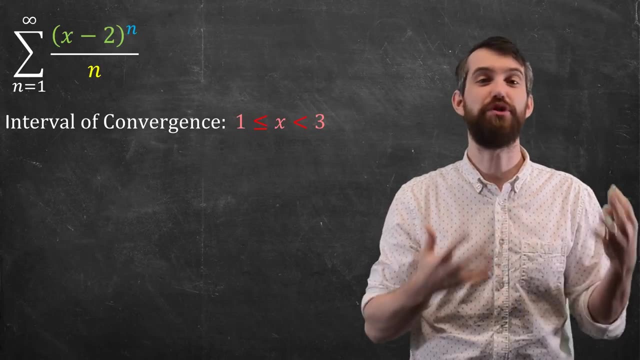 it diverged. The final answer: what do we have? Our interval of convergence is the one less than or equal to the x all the way up to the 3.. And other pieces of terminology I throw in the mix here- is that I will say that the radius of convergence is 1 and that the center of it is 2.. 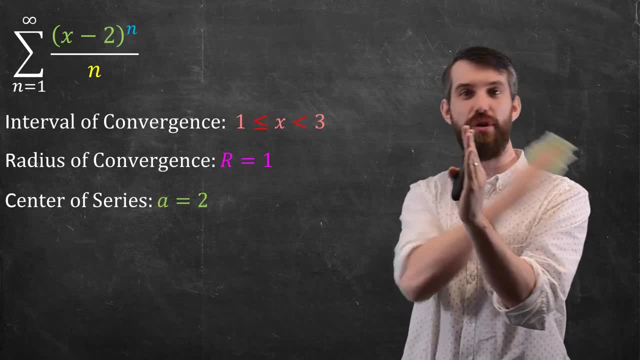 So I think of this 1 up to 3 as centered at 2, and then you can go off from the value of 1 on either side, So 1 up to 3, and then I've checked my endpoints, and one of them: 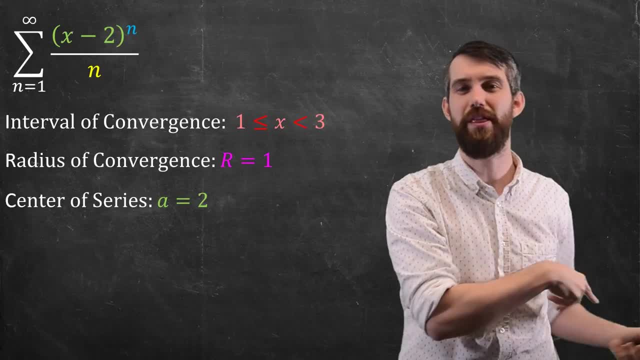 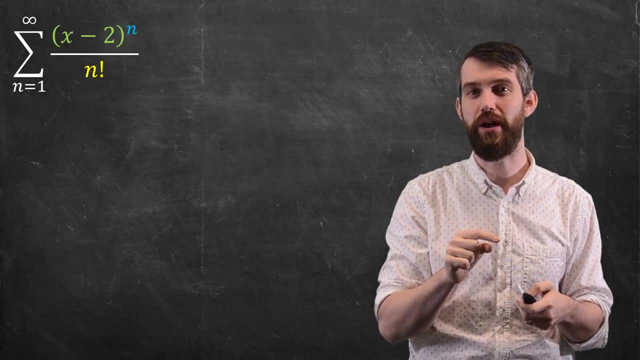 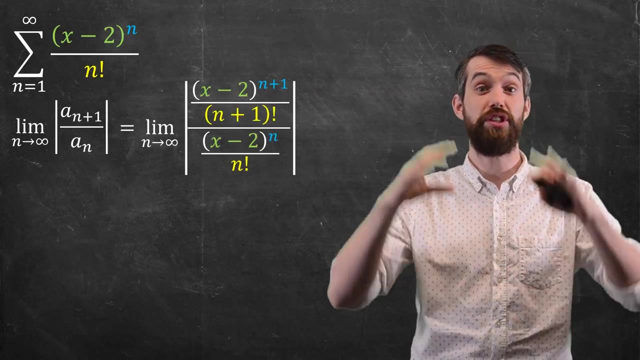 converged and one of them diverged. Let's see a couple other examples just to really lock this in. In this example, my cn- that constant sequence- is now 1 over n-factorial. So now if I do my ratio of the an-plus-1 over the an, I can have a much messier expression. First, the 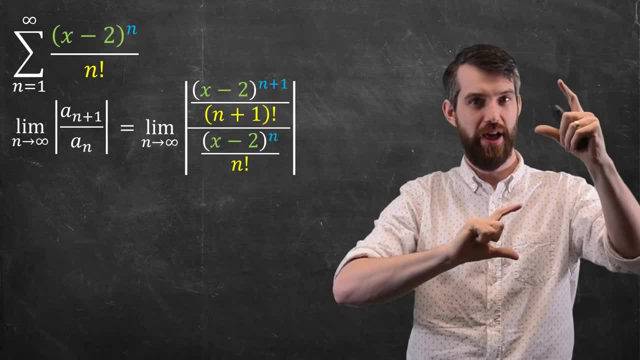 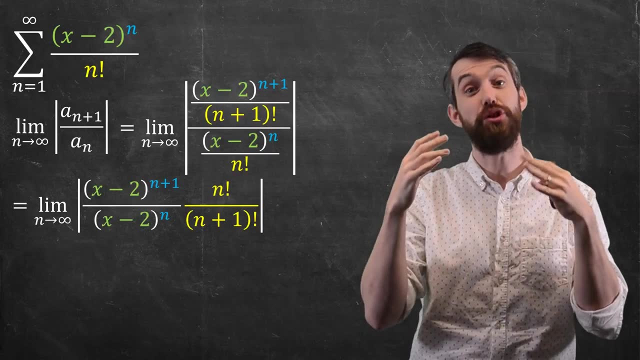 an-plus-1 termed on the top and the an on the bottom. If I bring the bottom up, then I get the following: x-2 to the n-plus-1 over an x-2 to the n, and then also this n-factorial over n-plus-1 factorial. Now the x-minus-2 part does the same thing, proof that x-2 and n-plus-1 are indigenous. 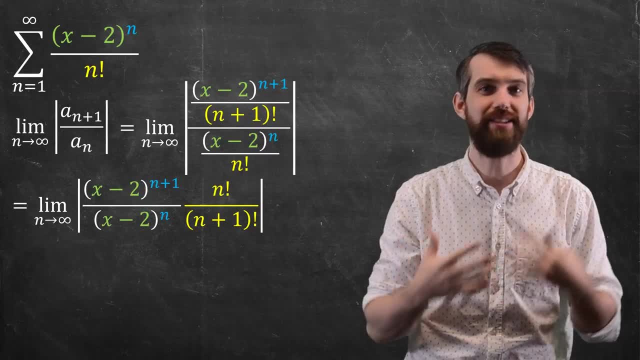 Well, I'm drawing a rectangle. I'm looking at the x-minus-2 to the n-plus-1 of the n-plus-1 over x-2 to the n. So what I'm? The x-2 part does the same thing. it just cancels and you're left with just a single copy of x-2,. 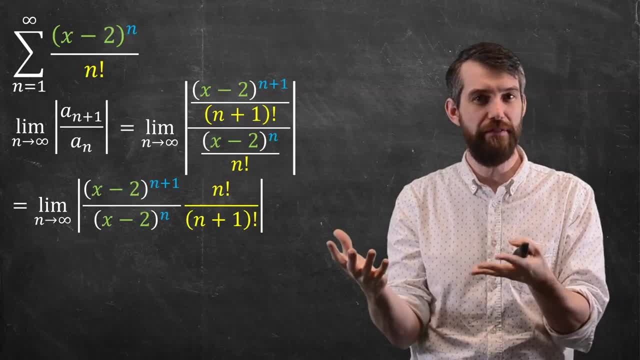 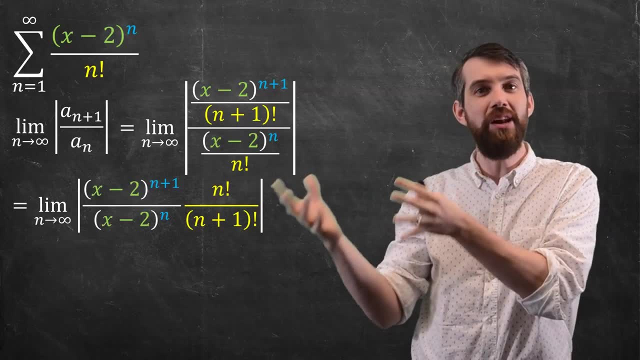 but let's think about the factorials. n plus 1 factorial is like n plus 1 times n times n minus 1 times n minus 2. all the way down It's kind of like n plus 1 times n factorial, So almost all. 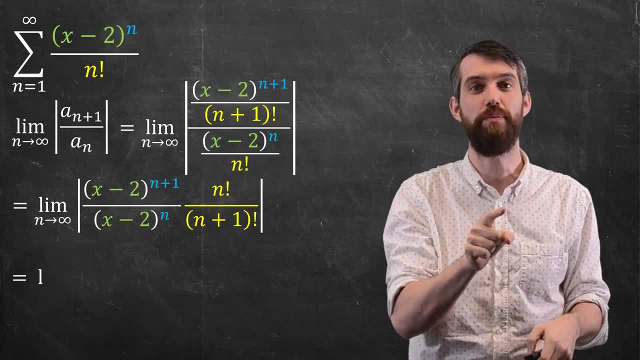 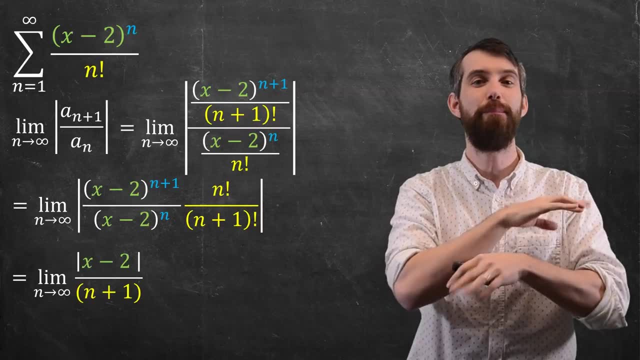 the terms in the factorial cancel, except the n plus 1 term by itself. and so what do I get? I get this absolute value of x minus 2 over the n plus 1.. Now it doesn't matter what x you put in here. you can put in x equal to a billion. the n will eventually drag it down and the limit goes. 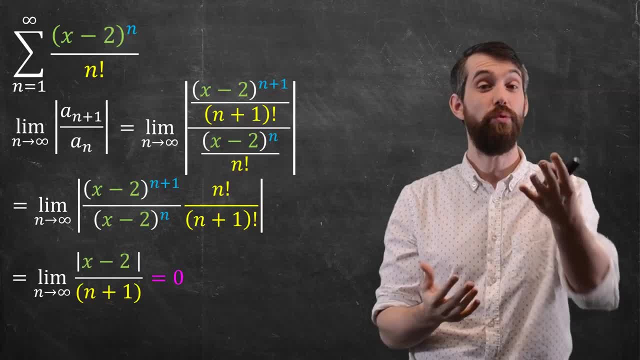 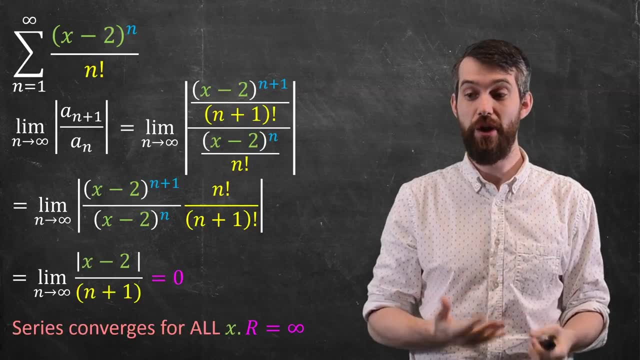 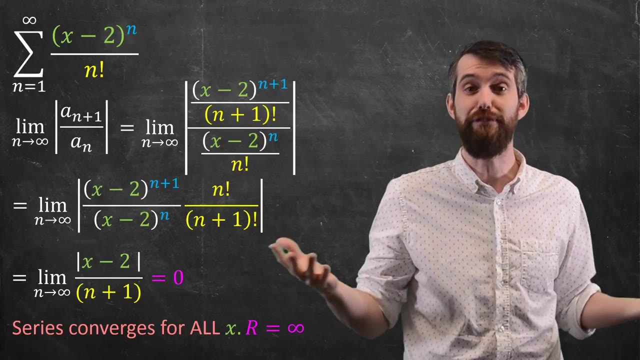 to infinity, so this limit is always 0.. So what the ratio test says is: because 0 is less than 1, is that this converges for every single value of x. and so we say our series converges for all values of x. and another way to think about this is that the radius of convergence is infinite. 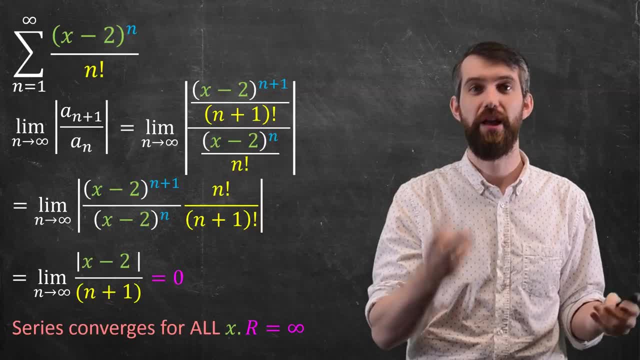 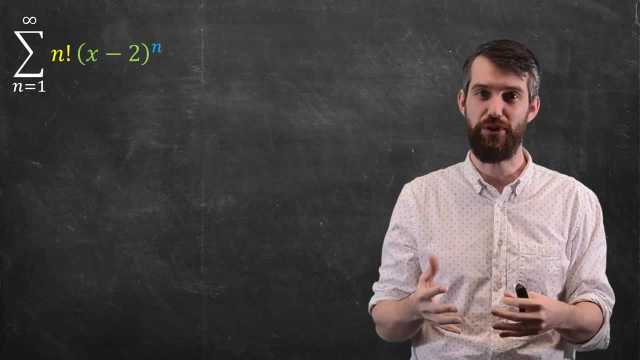 It's the interval from minus infinity to infinity. Third and final example: here now I'm going to take that n factorial. I'm going to move it up to the top. It's n factorial times the x minus 2 to the n. Again, I'm going to go and write down my 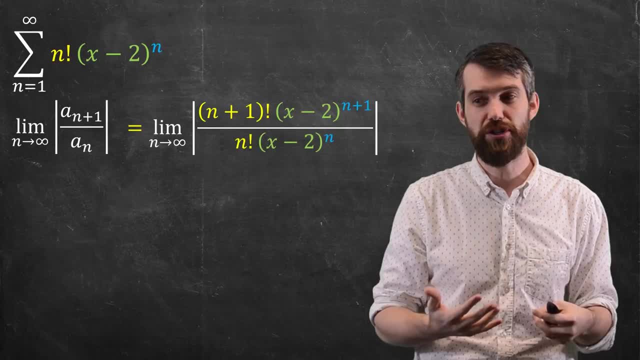 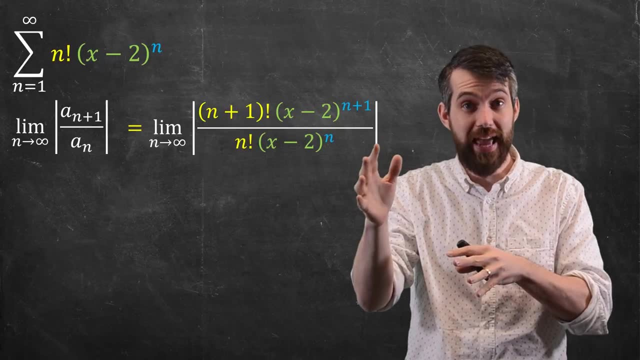 ratio test. I'll plug in the n plus 1 term and the n term Again. I get a lot of cancelling in my n plus 1 factorial over n factorial. Almost all of that cancels except the n plus 1 on the top. 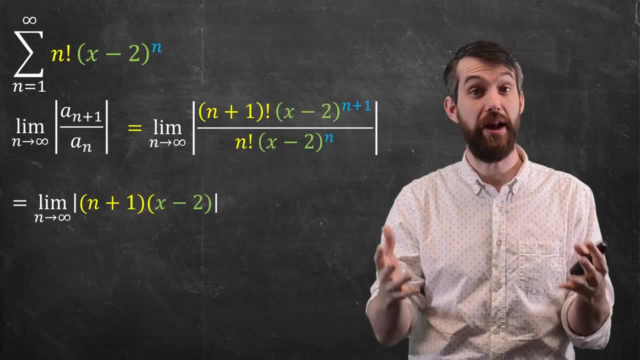 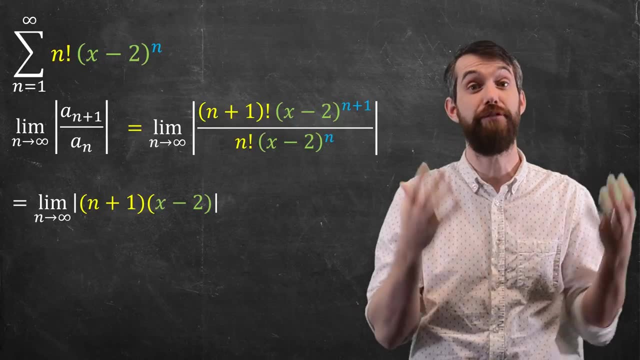 So what are I left with? n plus 1 times x minus 2.. Now this is, in general, going to blow up. That n term is going off to infinity and it's on the numerator, so it's going to get very large, Very large, that is, unless x is 2, in which case it's n plus 1. 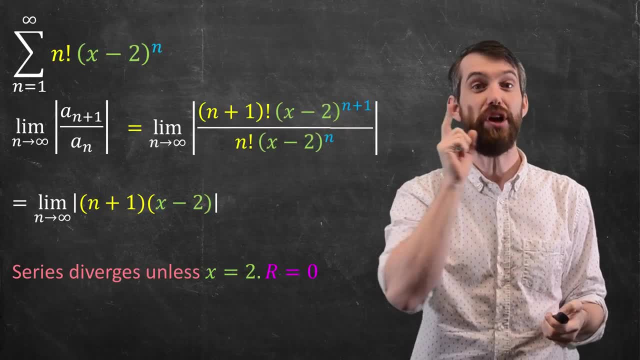 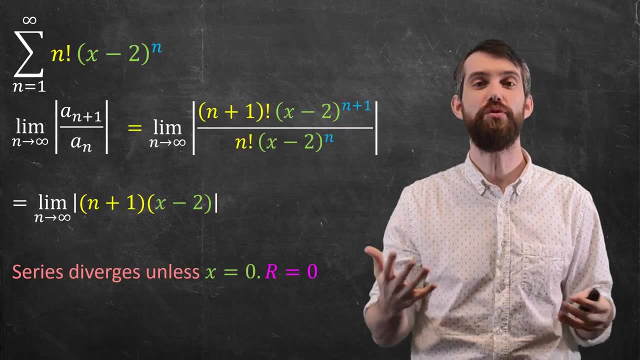 times 0, which is always going to be 0. So this converges only in that one case of x equal to 0, we say it is a radius of 0.. Now these three examples give us three different cases, three 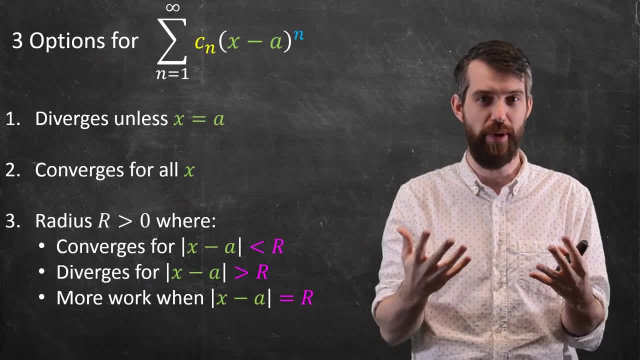 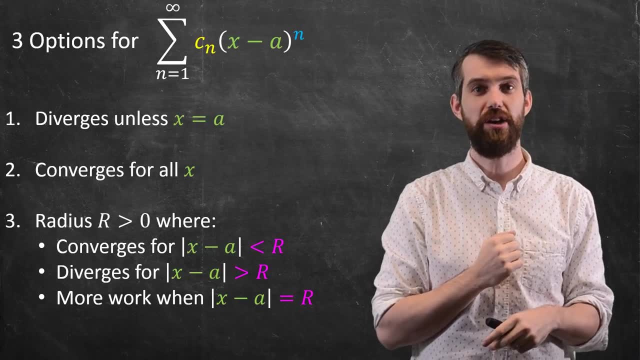 different possibilities, and in fact for a power series, these are the only possibilities. It could converge anywhere except for the x equal to a, the centre of your series. It could converge everywhere. That's a possibility too. or you could do what it did in the first example, where 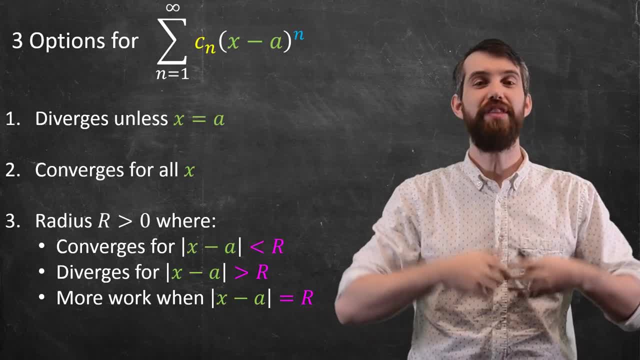 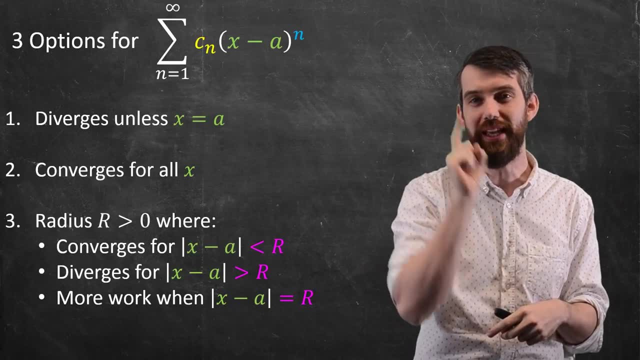 there was a radius of convergence where if the x minus a in its absolute values was less than the radius, it converged, If it was more than it, it diverged, and if it was equal to it then you had to go and plug in the values and adjudicate what happened in that. 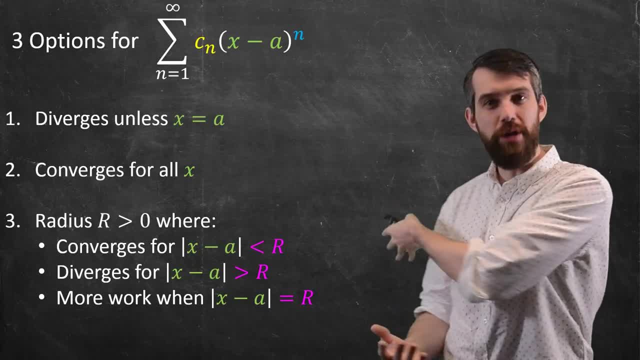 final fringe case. So have a power series. one of those three possibilities will occur and you apply the ratio test to try to decide which case are you in.